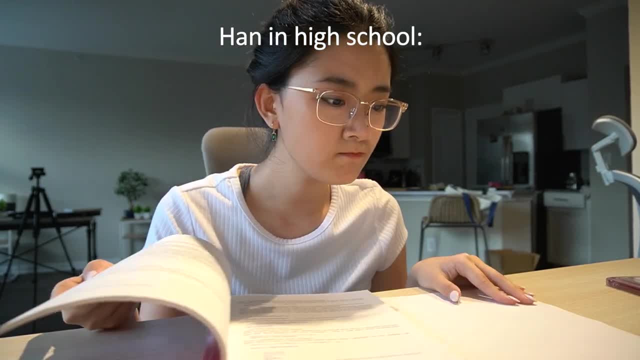 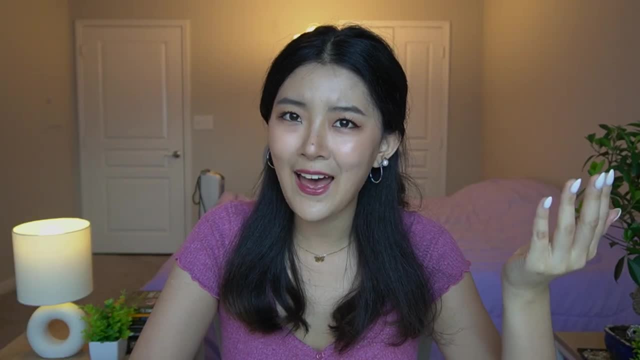 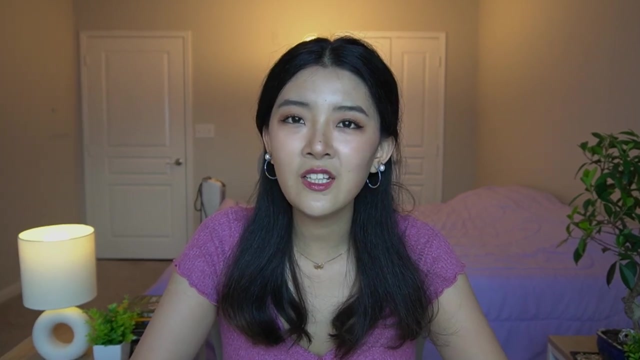 I spent hours looking at how to solve different math problems, going over each problem carefully to see how it's done. You may stop me and be like hold on, that doesn't sound bad, Sounds like you are a hard worker, But if you pay close attention, the problem here is it's solely passive learning. 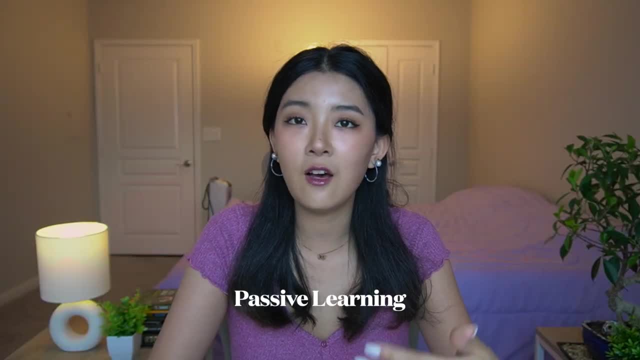 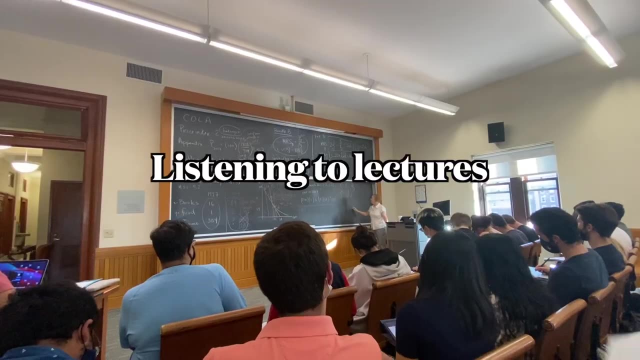 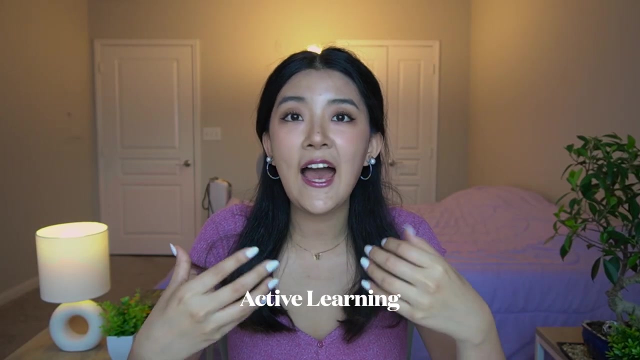 and no active learning at all. Passive learning is a method of learning where students receive information from outside sources and try to internalize it, which include listening to lectures, reading and watching demonstrations. And active learning means you are actively involved in the learning process. Basically means that you are doing something besides just. 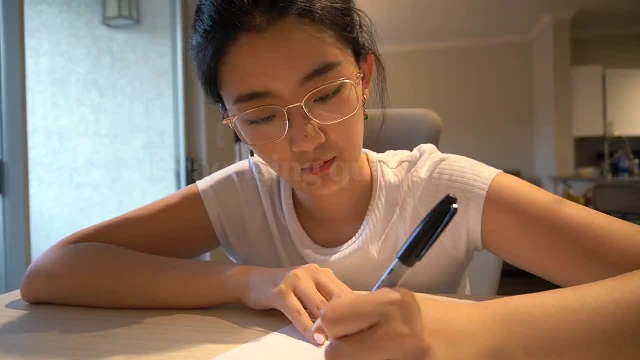 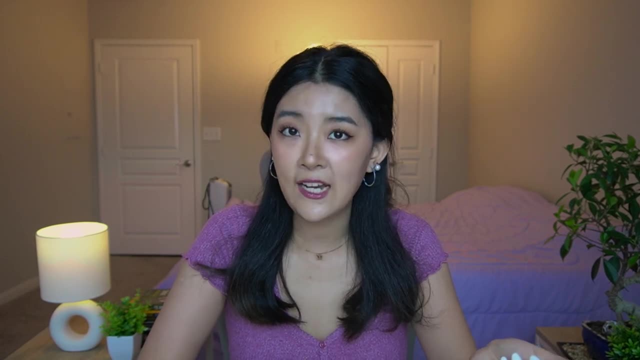 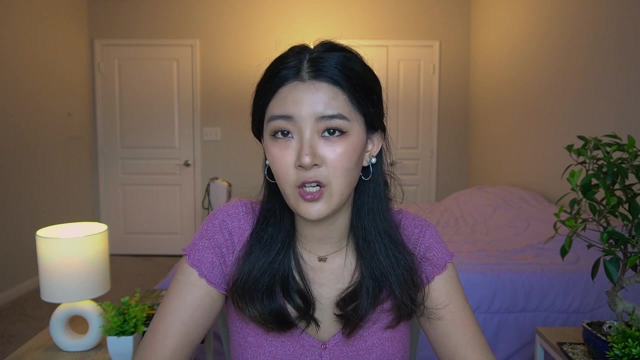 receiving the information, which includes discussions, practicing questions and teaching others. In our education system, there are lots of passive learning and very little active learning. Many research studies have shown that passive learning is not as effective as active learning in math and science education. So if you feel like you're spending lots of time in studying math, 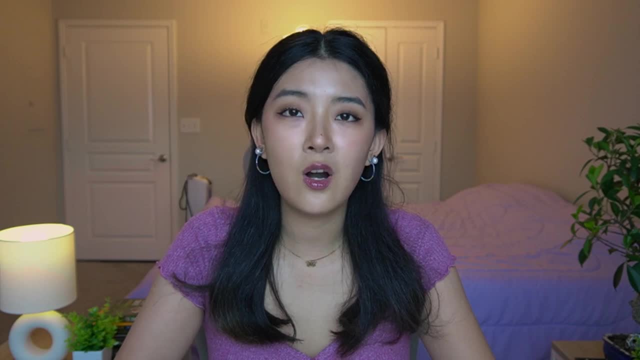 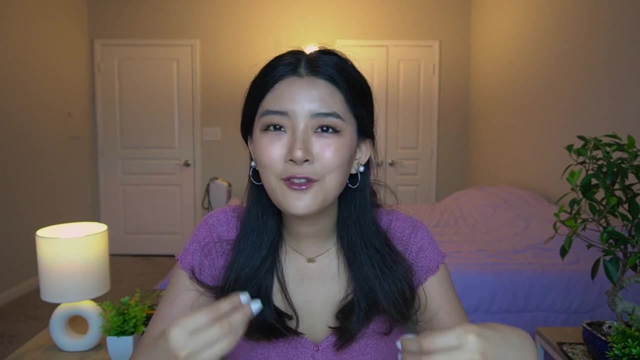 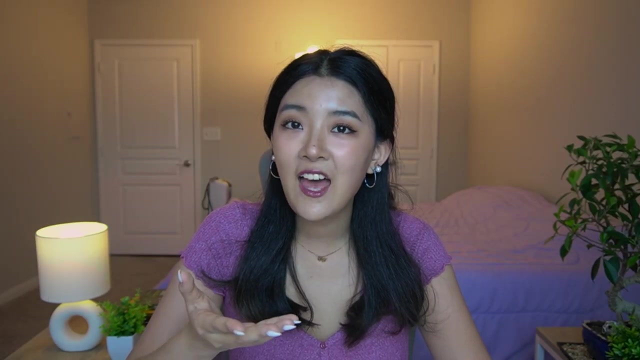 but still not get good results. it's probably because you are doing too much passive learning in math. Math is a skill to help you solve problems. You have to know how to use it. by doing it, You wouldn't say that you can drive a car just by watching someone else drive. and 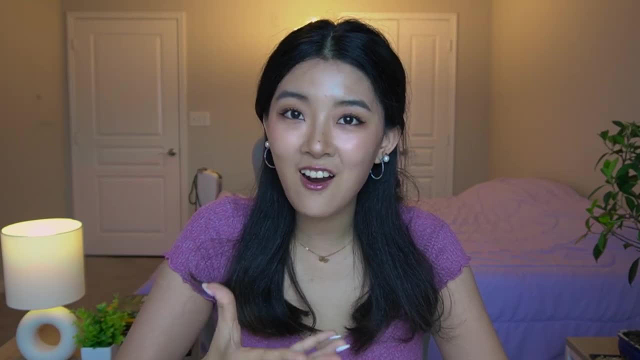 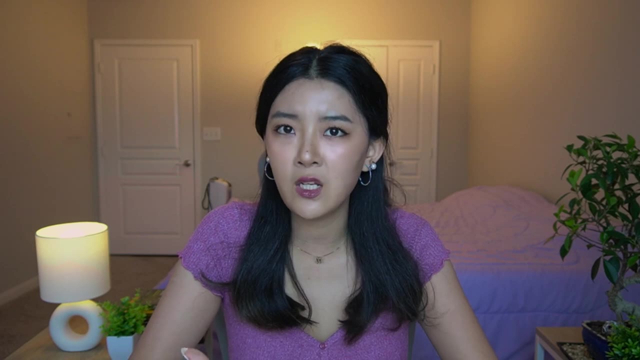 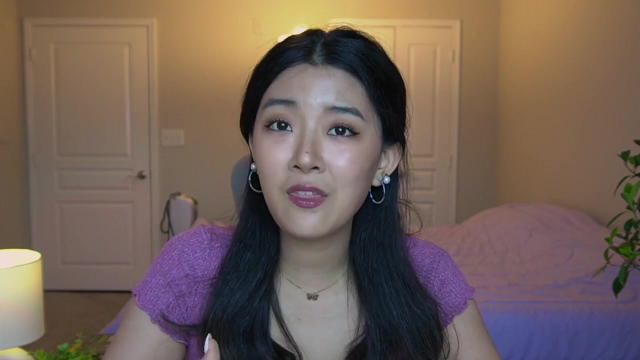 memorizing all the traffic rules. You have to get into the car and practice. This way you can know how it feels, which part you have problems or any complications you may run into. So I hate to break this to you, but if you only read and listen how the math is done, 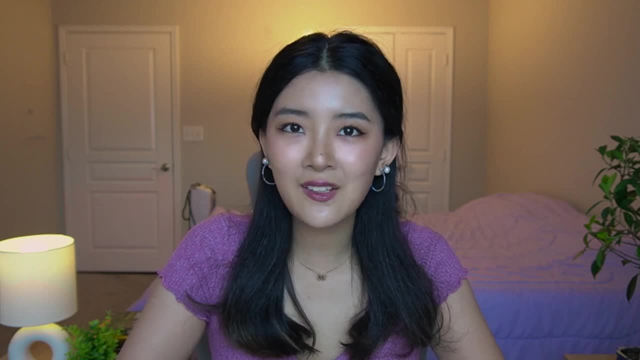 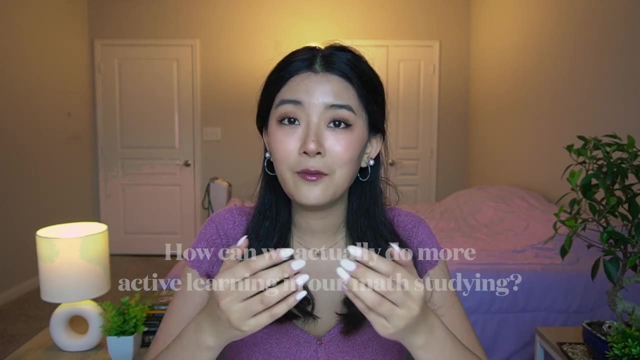 sometimes you may think, oh, I understand the math, but actually you don't. So how can we actually do more active learning in our math study? If there's one thing I wish you can take away from this video is, if you get a question wrong, always redo it independently. 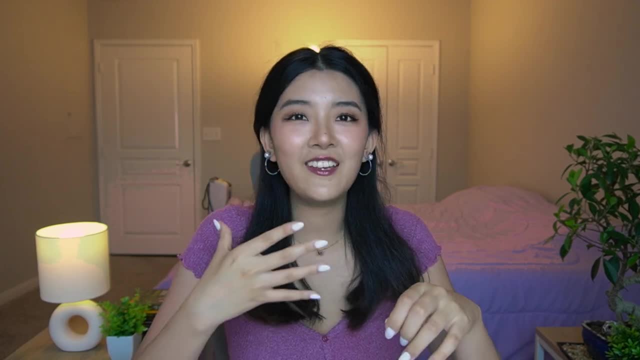 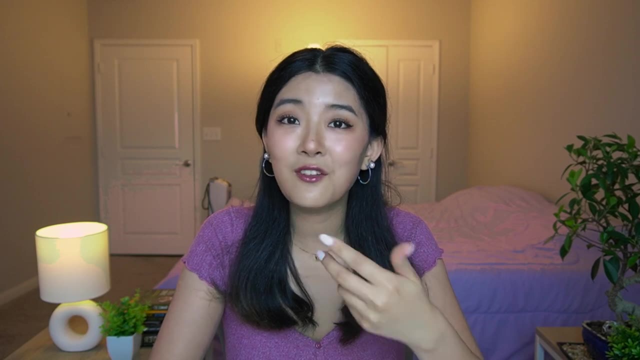 until you get it right. Lots of times people get really upset when they get a question wrong and start thinking: oh, what is wrong with me? I just cannot understand why I cannot do math. You know what The question in front of you is literally telling. 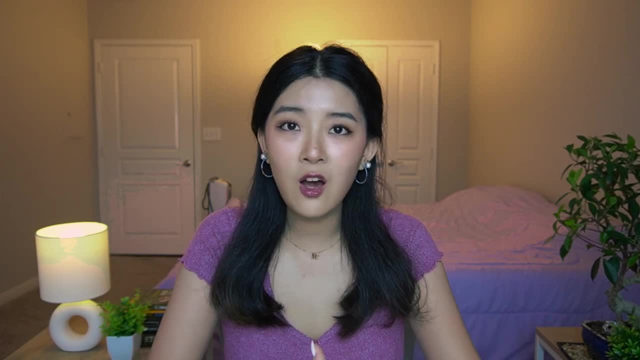 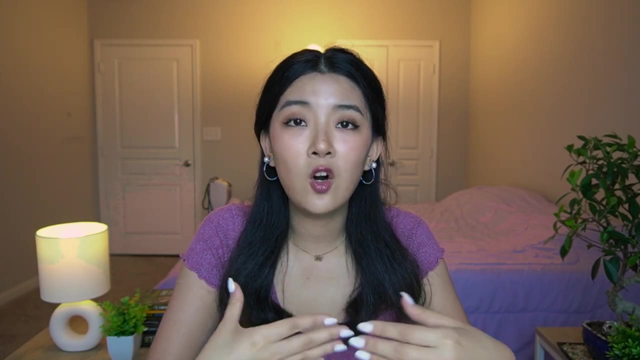 you what's wrong. What I often did was, if I got a question wrong, I just read through the answers and try to understand it and just move on. But again, the problem here is if I only read the solutions and try to understand how it's done. 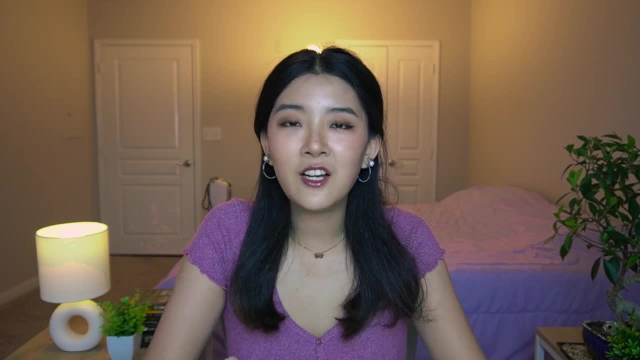 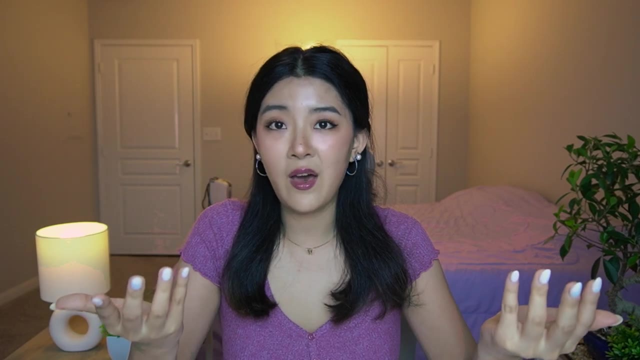 it's still a form of passive learning. You wouldn't go to the doctor, spend two days doing all the lab work for a physical exam and receiving a result that says you have a heart issue, and you just go. oh crap, they say I have a heart issue and just move. 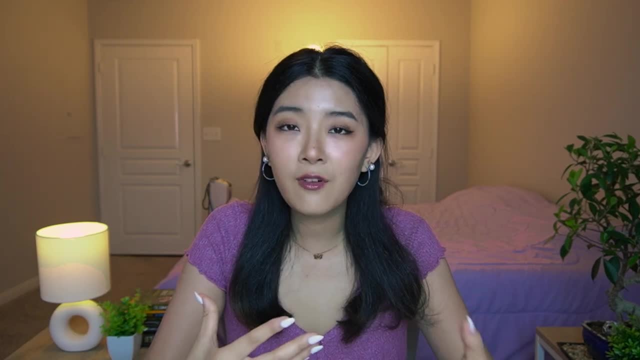 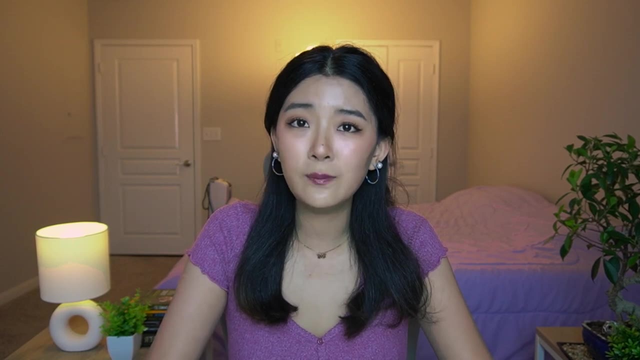 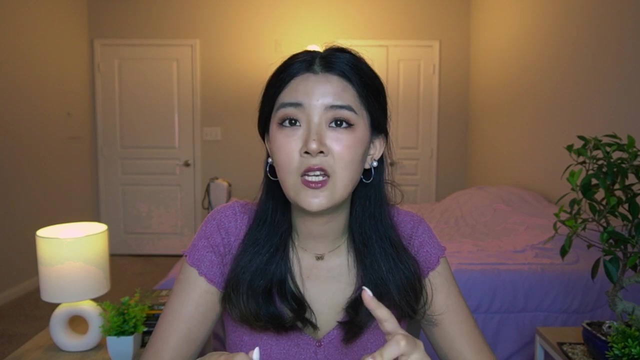 life. You would actually follow up with the doctor, take pills every day or pursue whatever the necessary treatment it is until the disease is cured or under control. Every time you practice a question, it's a diagnostic process to see whether you understand the math concept and your 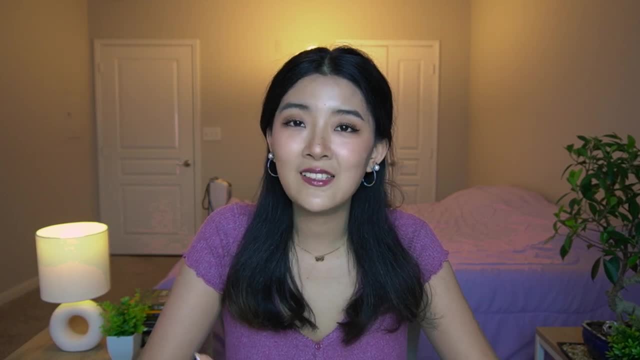 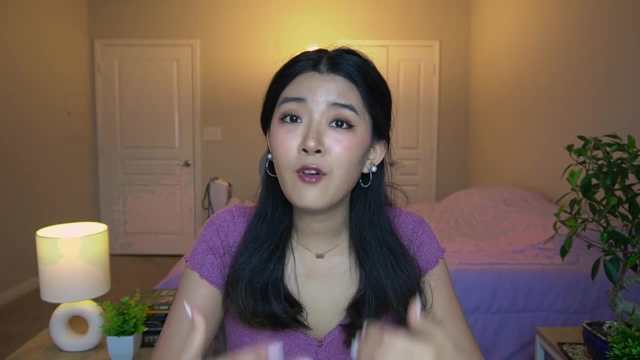 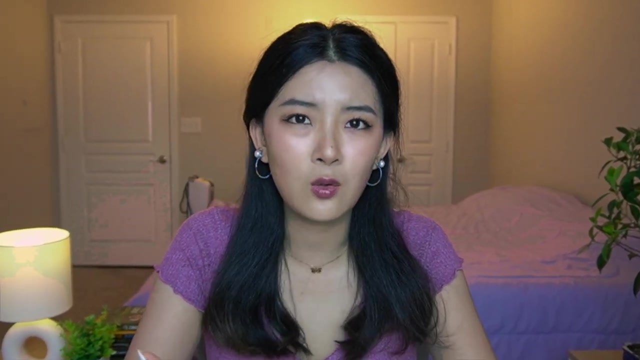 ability to solve the questions, And you need to realize that the diagnosis is not the most important part, and what truly matters is the treatment. You've already invested all your time and efforts in reading the question, trying to understand the question, thinking about the 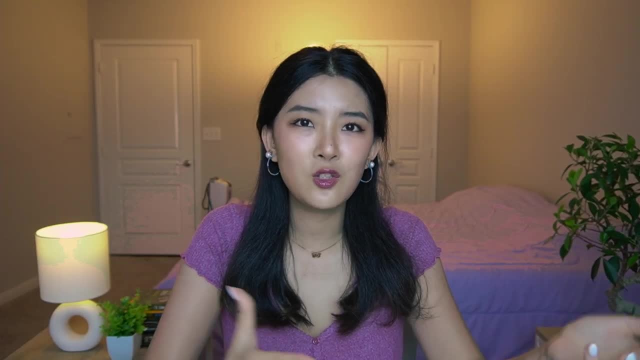 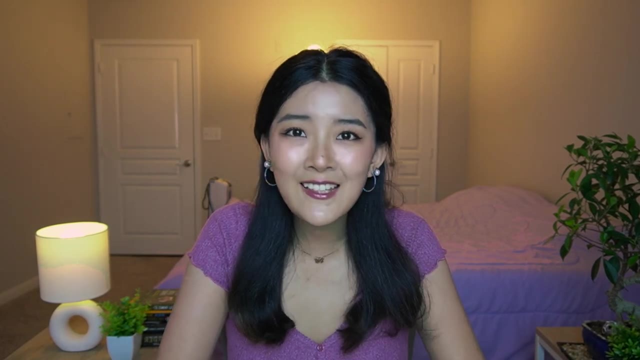 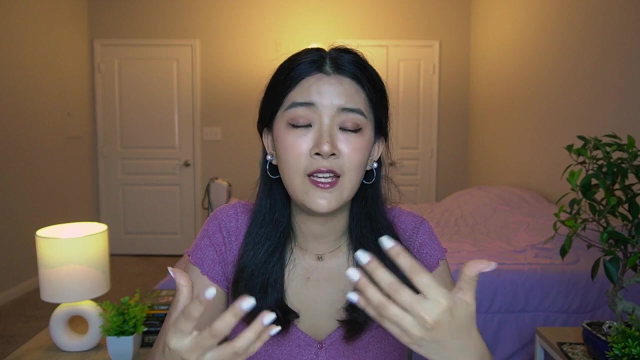 question: write the question. If you don't follow up with what's wrong, it's really just a waste of time. So follow up with the question that's wrong. figure out precisely which step you made a mistake, really trying to understand why you made that mistake and how you can prevent it from happening. 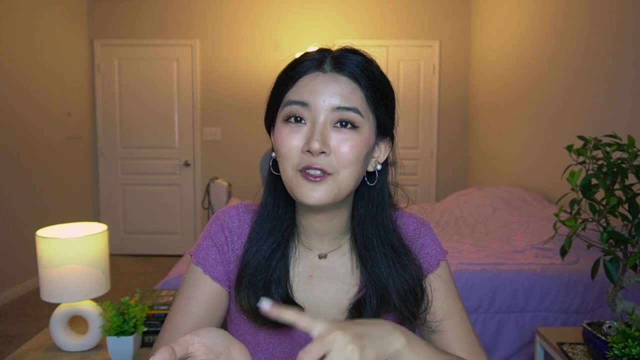 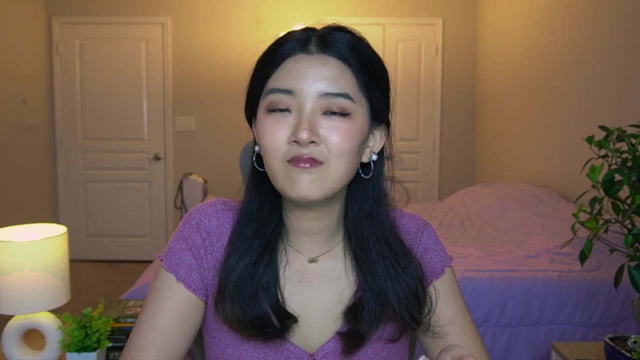 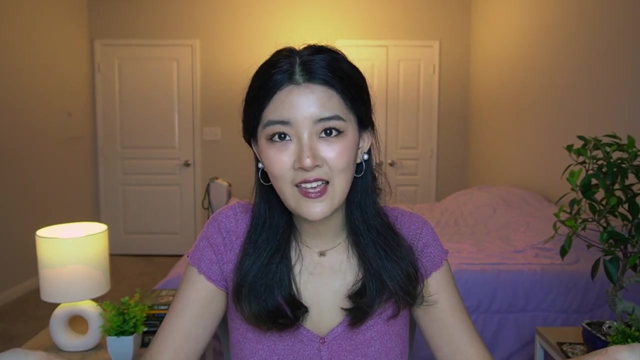 in your life And doing the question again: is the follow-up doctor appointment that they will tell you whether the disease is truly cured or not? Because the doctor may tell you, yeah, you know what, you're good to go. Or they may tell you it's still there, you still haven't fixed it. Or they may even say: 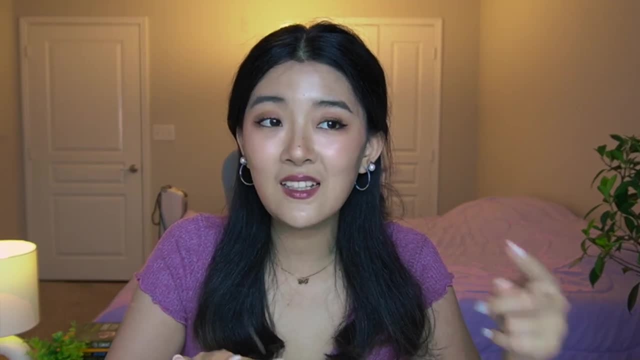 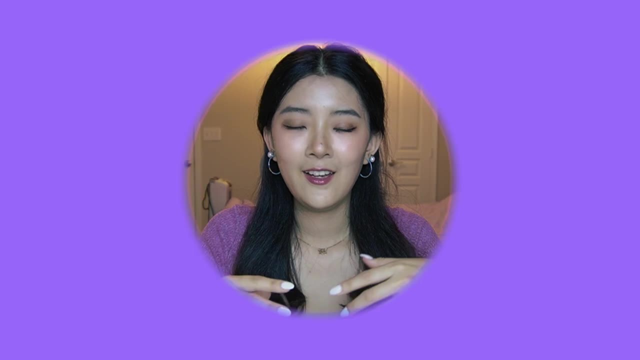 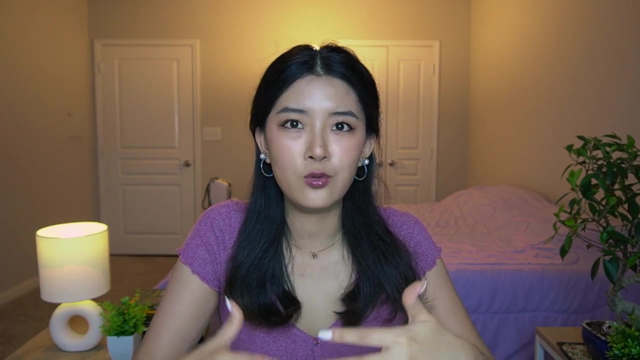 that, ah, your heart disease is cured, but now you have a liver disease. So make sure you test yourself by doing the questions again until you get it right. So how do you actually follow up with your math disease and then find the treatment for it, aka how to fix the problem? 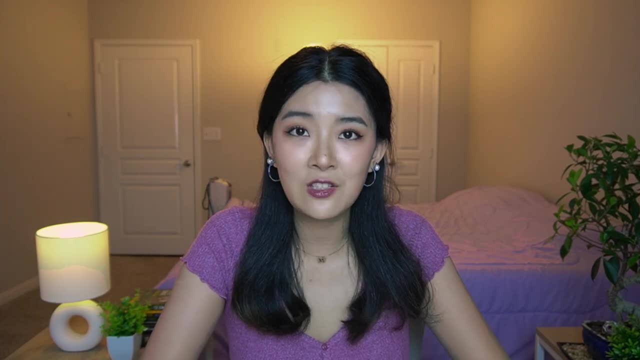 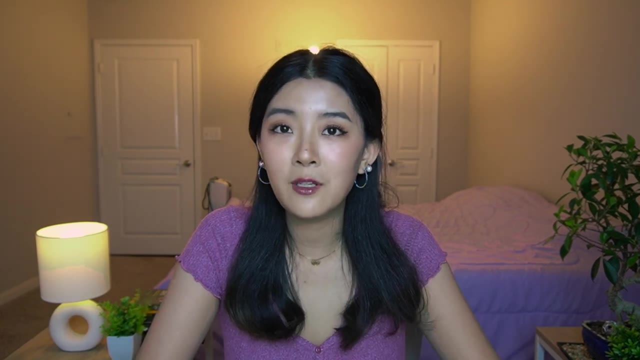 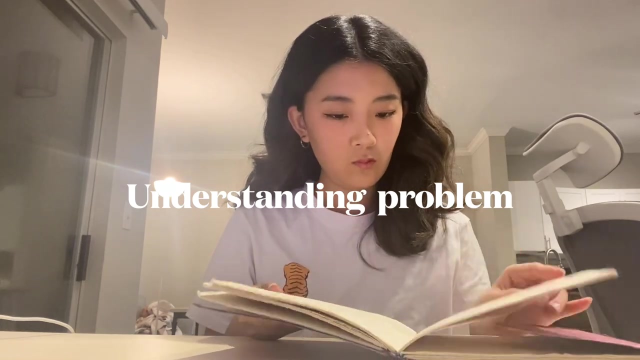 So essentially, you compare your wrong answer to the correct answer and figure out which exact step that you had the problem. In my experience, there are four types of problems. Let's just dive into each one of those. Firstly, an understanding problem might arise when you fail to grasp a math. 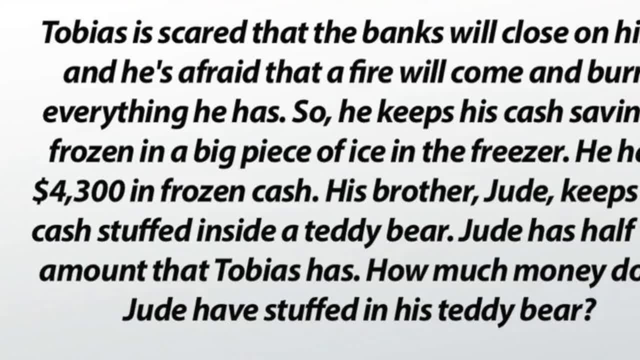 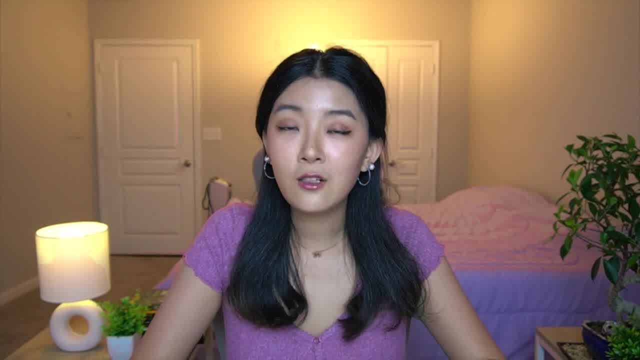 concept or the equation you recently learned, or perhaps you don't understand the question itself. To help you understand math better, consider using the Feynman technique. It is a learning method that is used by the Nobel Prize winning physicist, Richard Feynman. Basically, 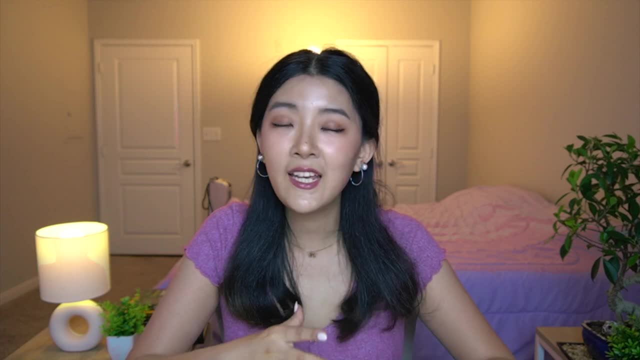 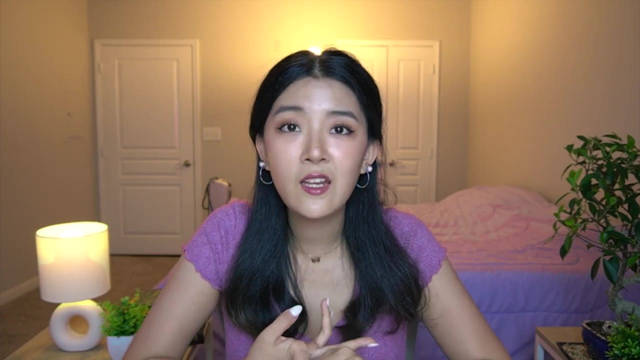 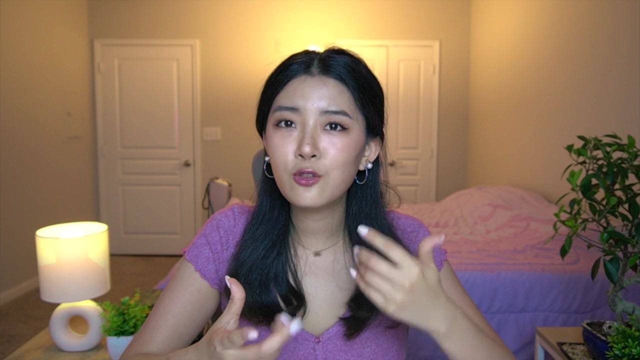 the way you understand a concept is by explaining it, as if you're explaining it to a child. While doing this, notice which part did you struggle to explain? what details did you miss? what part is really hard for you to put into simple words? Answering those questions will show you which. 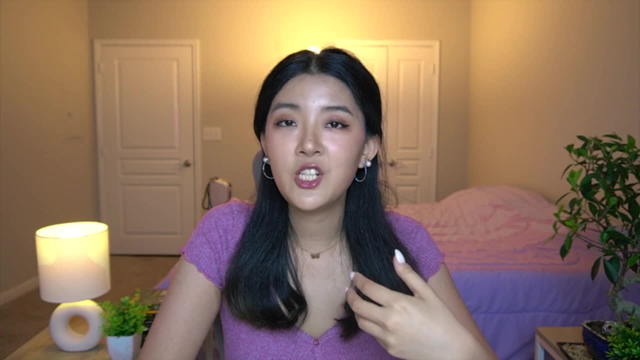 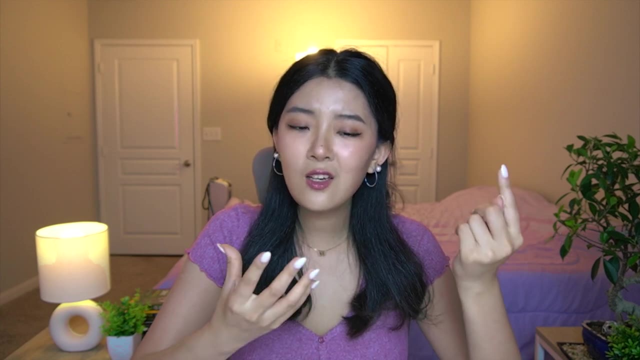 part are you missing? The act of explaining to yourself or teaching others is a form of active learning. Sometimes, when we're thinking about things in our own mind, we think we understand it well, but we may miss some important stuff. So the best way to uncovering those details? 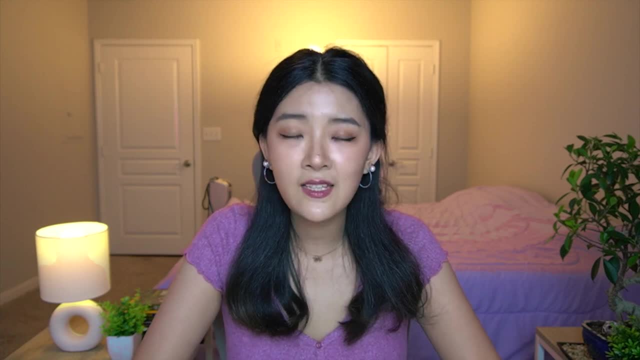 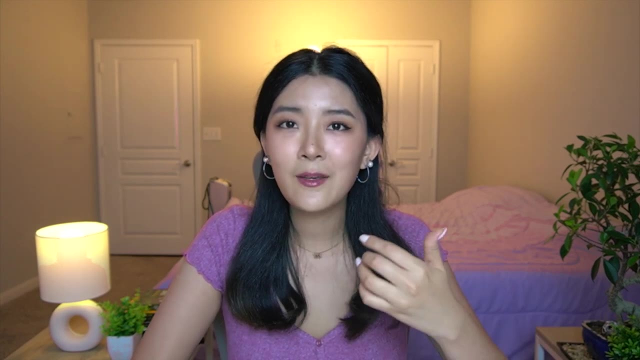 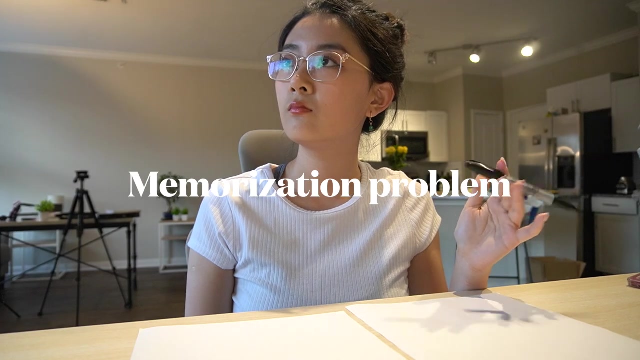 is to explaining it out loud, verbalize it and teaching someone else who doesn't know about the topic. And the more you can put it into simple terms, the better understanding you have about the topic. Secondly, you might face issues with memorization when you can't remember an equation function. 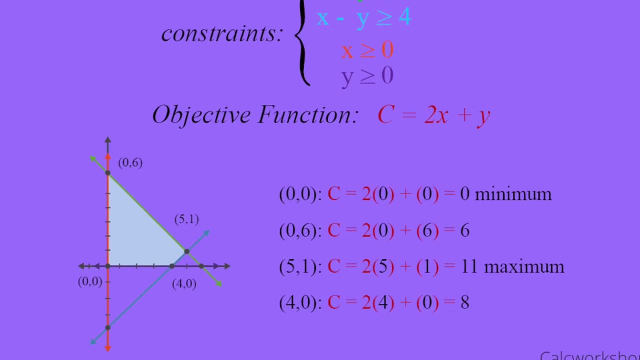 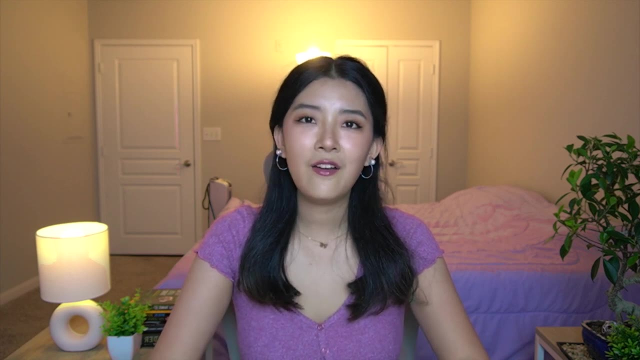 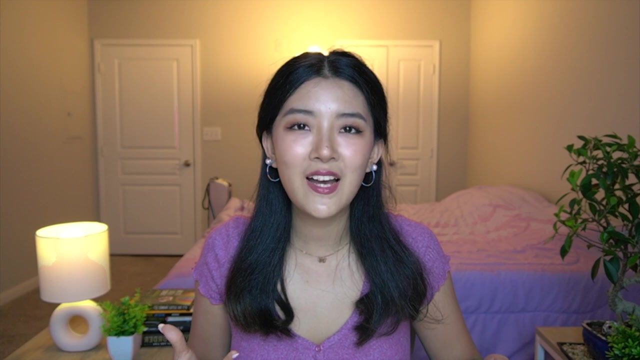 or the specific steps required to solve a particular type of problem. In my opinion, in math memorization is really often unnecessary, because everything can be proven. If you're really motivated not to memorize anything, you don't even need to memorize. 1 plus 1 equals 2, because 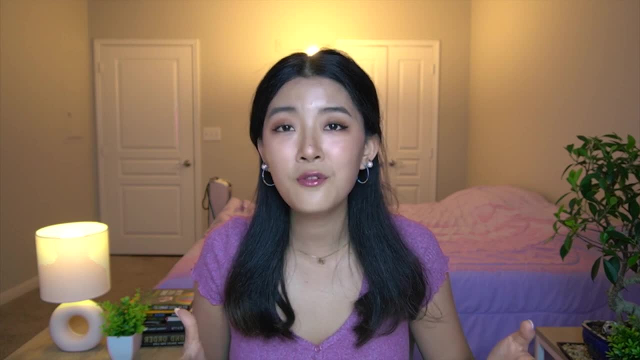 there are 162 pages of proofs in the book. So if you're really motivated not to memorize anything, you don't even need to memorize. 1 plus 1 equals 2, because there are 162 pages of proofs in the book. 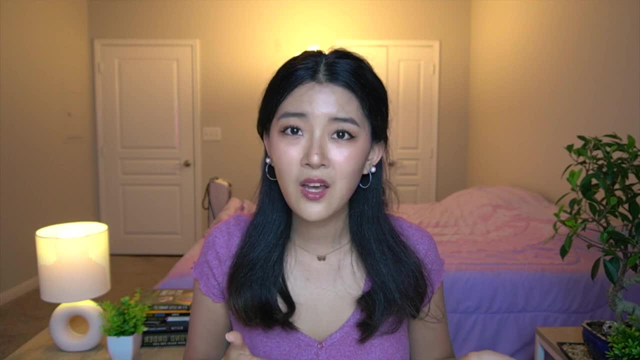 So if you're really motivated not to memorize anything, you don't even need to memorize. 1 plus 1 equals 2, because there is an abstract algebra to prove why 1 plus 1 equals 2.. Therefore, I highly recommend you try to understand everything before. 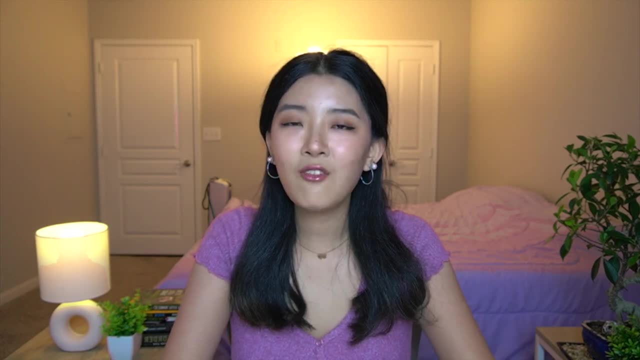 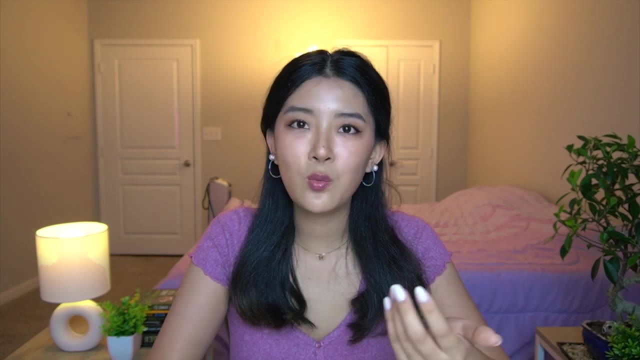 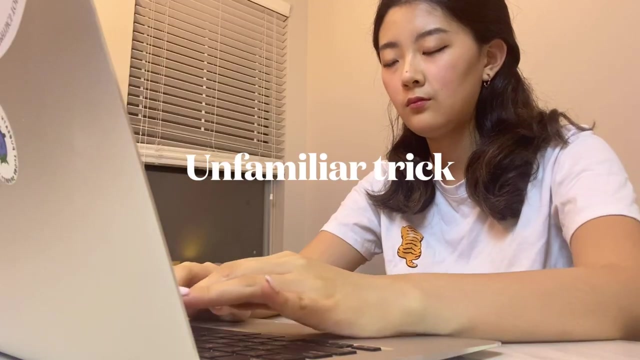 you just straight jump into memorization. But in our daily math studying memorization does have an important role because it really can save us time. In situations where memorization is necessary, the best technique is active recall and spaced repetition. Third, some questions may need a.